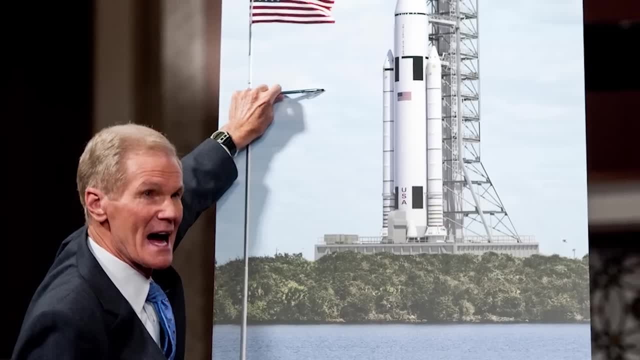 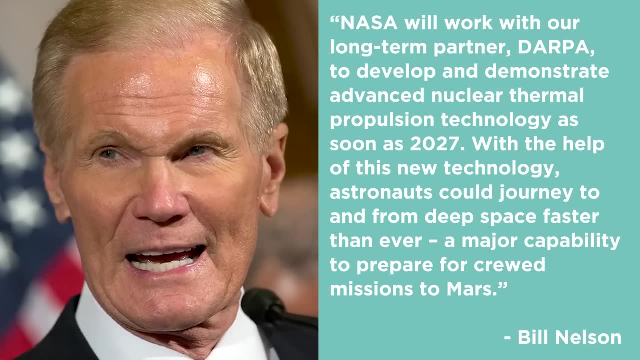 Yeah, there's a gonna be some acronyms up in here. NASA Administrator Bill Nelson summed up the program like this quote: NASA will work with our long-term partner DARPA to develop and demonstrate advanced nuclear thermal propulsion technology as soon as 2027.. 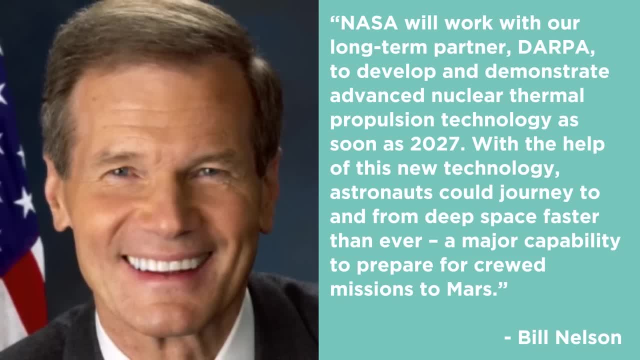 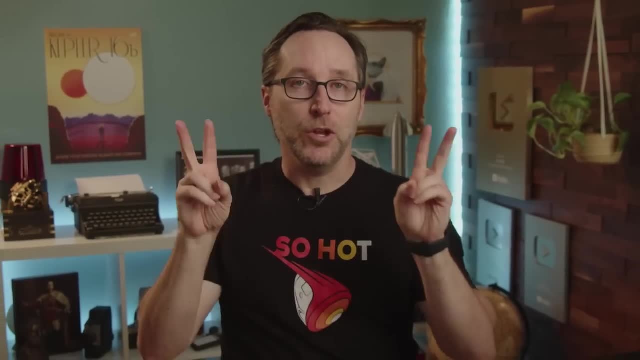 With the help of this new technology, astronauts could journey to and from deep space faster than ever, a major capability to prepare for crewed missions to Mars. The part of that announcement that makes space nerds all tingly is the nuclear thermal propulsion part of it. 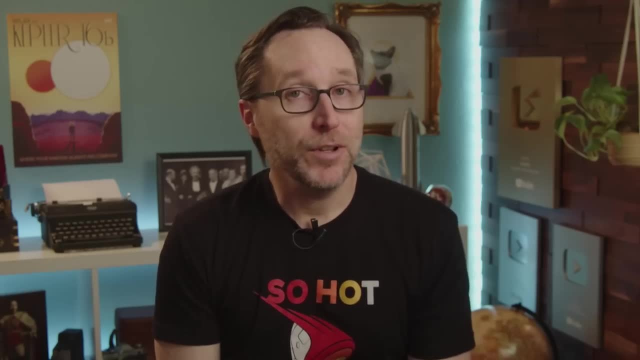 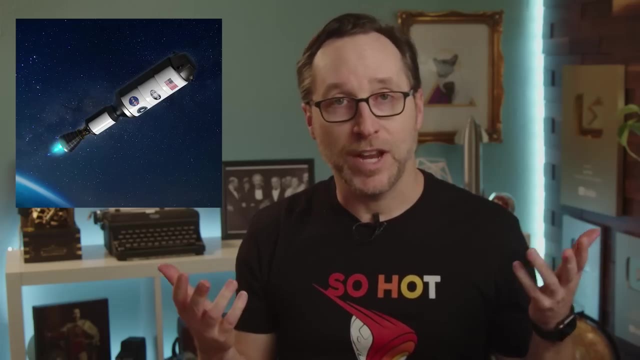 So, yes, finally, at long last, NASA's building a nuclear rocket, And the timeline is ambitious, if not completely ridiculous. Because not only are they wanting to get an entirely new type of engine up and flying in five years, DRACO will include a rocket, a spacecraft and a launch vehicle. 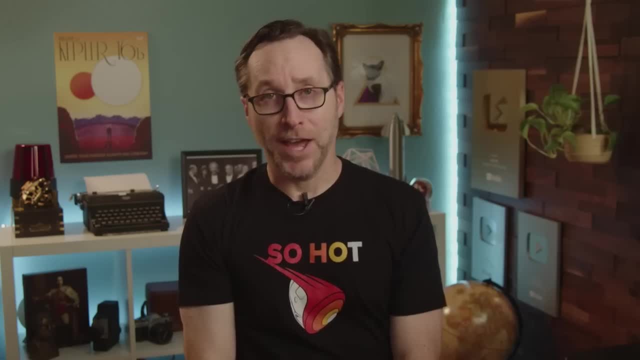 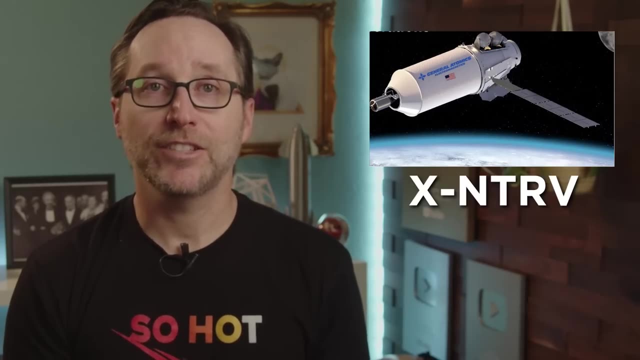 All by the end of September 2027.. Good luck with that. The spacecraft has a name and of course it's an acronym: the Experimental Nuclear Thermal Rocket Vehicle, or EXENTERV- Swinging a mess on that one- And these nuclear engines will be powered by a type of fuel. 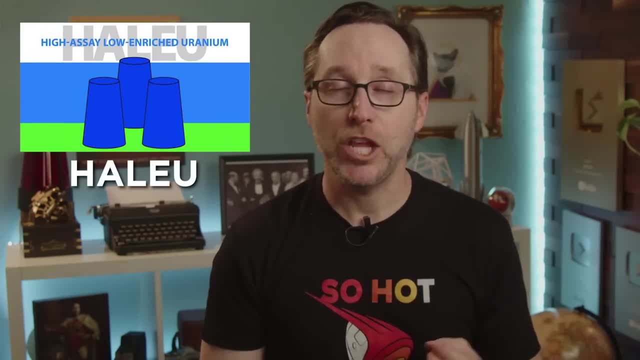 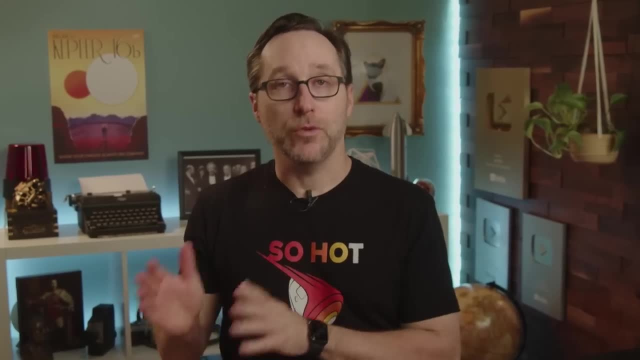 called High-Assay Low-Enriched Uranium or HAL-E-U, HAL-E-U, HAL-E-U, HAL-E-U, HAL-E-U. Never know how to pronounce that The low-enriched uranium part isn't anything special. that's what most nuclear power plants use. It's the high-assay part that sets it apart. Assay is basically the concentration of fissile isotopes, so higher assay means more bang for the buck. So HAL-E-U fuel has an assay between 5 and 20% of fuel mass. 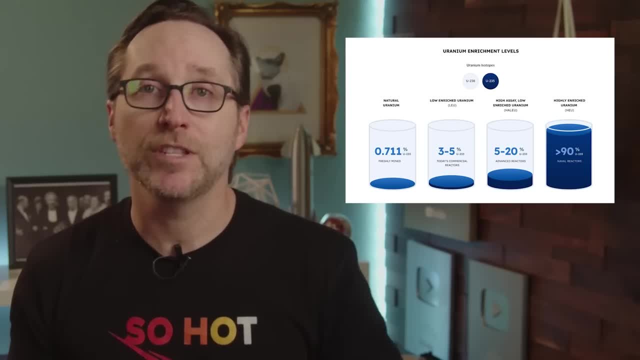 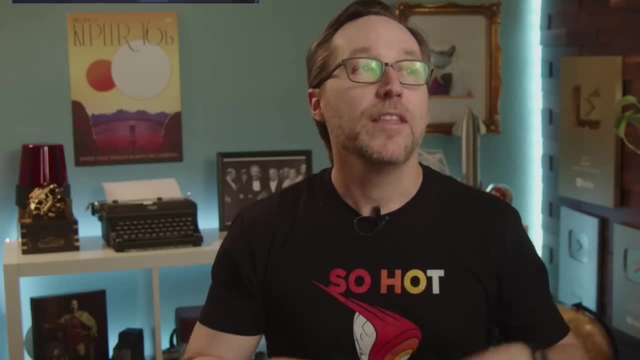 That's much lower than, say, the 90% plus used in nuclear weapons, But it's higher than the assay of uranium used in power plants. I actually talked about HAL-E-U in a previous video about uses for nuclear waste. There are some experimental reactors out there that can make this out of nuclear waste. 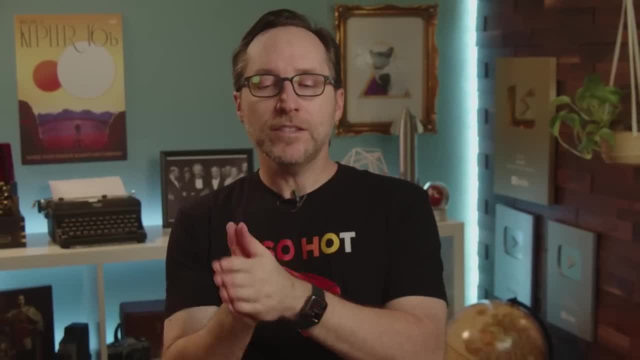 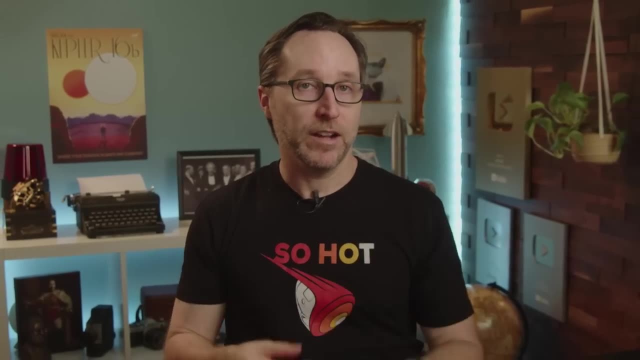 and then use that to make energy with it. Okay, so why is this such a big deal? Why is this such a step up from the chemical rockets that we use now? So, for one thing, it doesn't require an oxidizer like chemical rockets do. Okay, so stepping back, just in case there's any like total rocket noobs out there. So, uh, rocket fuel needs oxygen to burn, Just like everything on Earth. The problem is that rockets leave Earth. That's kind of the point. 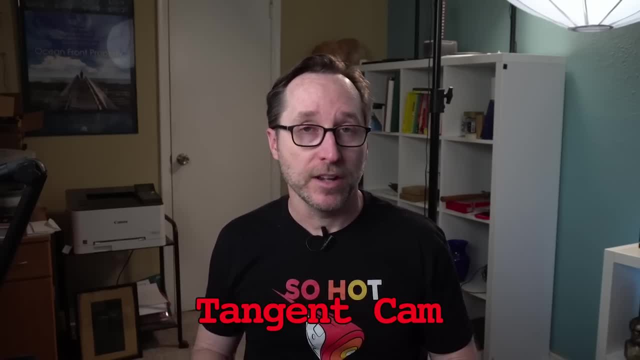 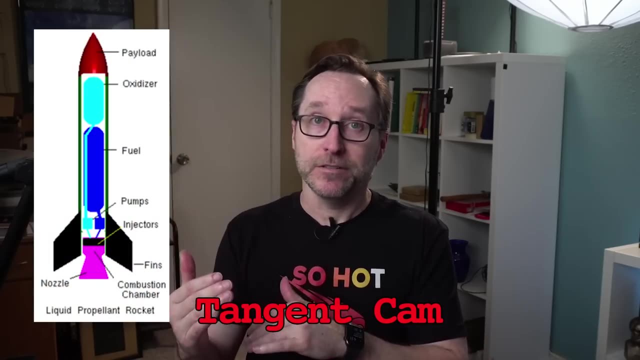 So rockets have to bring their oxygen with them in the form of liquid oxygen. So like big rocket tanks, like the SLS, when you look at that, that's actually only half fuel. The other half is oxidizer. This not only adds a lot of weight, it also cuts down on the amount of time that the rockets can burn, because you're literally emptying two tanks at once. But a nuclear rocket doesn't need oxidizer because it's not actually burning the fuel. It's just just kind of using that nuclear fission to superheat it and expand it. 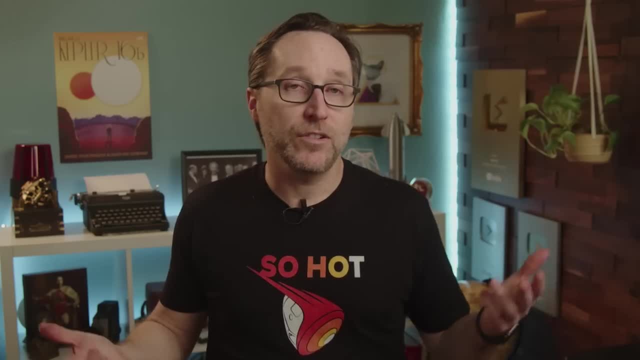 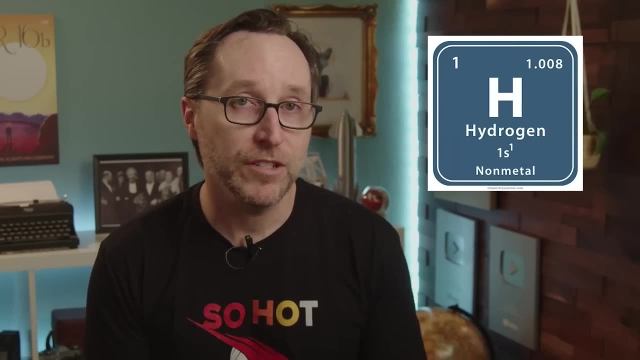 which flings it out the back and gives it thrust, And without all that oxidizer, those nuclear rockets save a ton of weight, Actually many tons of weight. Most nuclear rocket designs use hydrogen as the fuel of choice because of its low atomic weight. Um, there are some downsides to this, though, Because, yeah, nuclear rockets save mass on oxidizer, but past designs have needed at least three times the amount of hydrogen to create the same thrust. It's too early to say that that's the case with Draco, though. But to get back into the plus, nuclear rockets have a very high specific impulse, which means they are super efficient. Specific impulse measures how efficiently an engine converts fuel to thrust. This is often measured in seconds, as in how many seconds it can create thrust in Earth gravity. 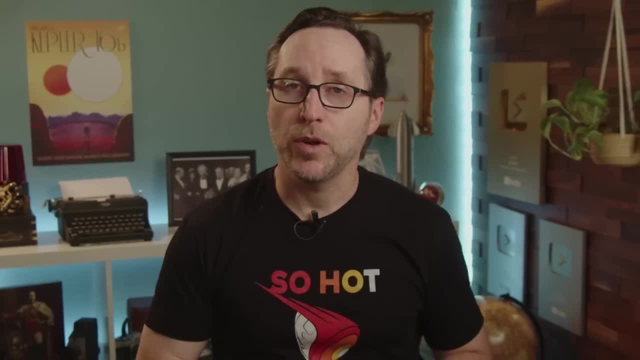 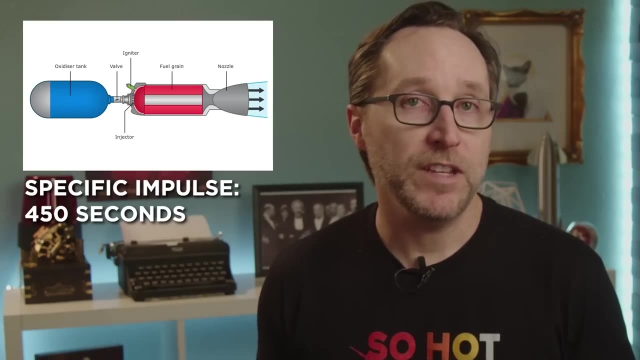 And according to an article from the US Office of Nuclear Energy, in December 2021, the initial target for a nuclear-powered rocket would be twice as efficient as chemical rockets, Chemical rockets having roughly 450 seconds of specific impulse, meaning the nuclear rocket would have around 900 seconds. 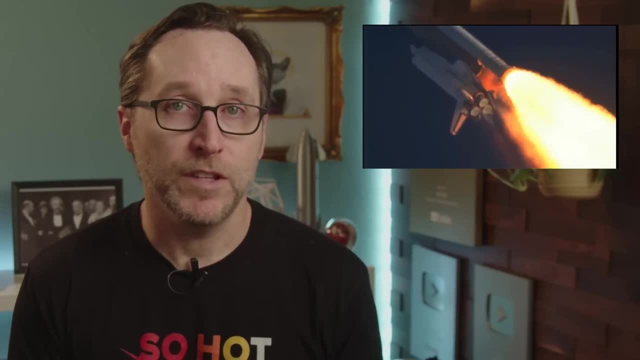 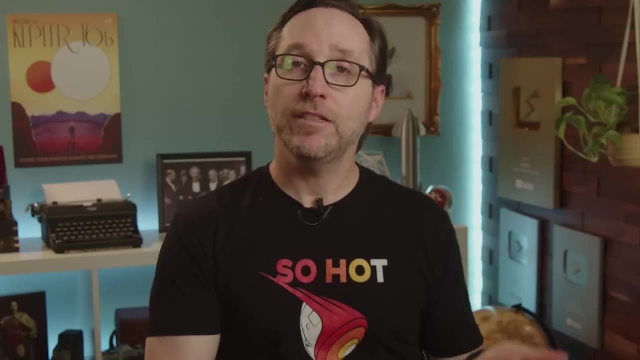 So, for example, the space shuttle had a specific impulse of just over 450 seconds, which is about seven and a half minutes. An engine powered by a nuclear rocket would be more like 15 minutes, And the longer you accelerate, the faster you can go. 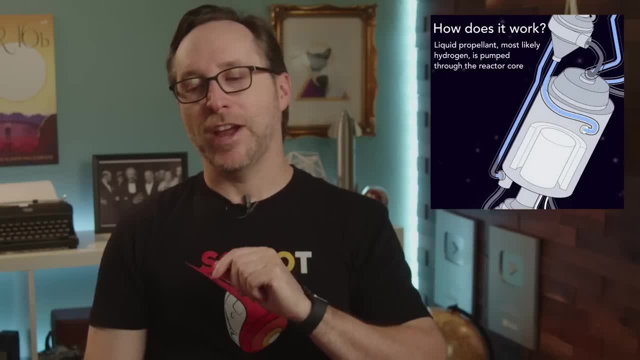 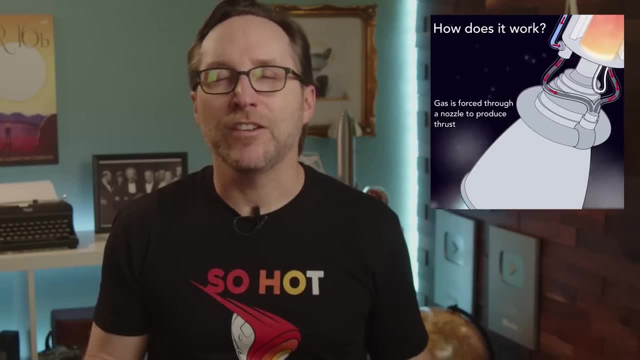 That's kind of the idea behind ion drives And, just like ion drives, we won't actually be seeing these being used to get off the ground. They're just for once we're in space. You can kind of think of these as ion drives on steroids. 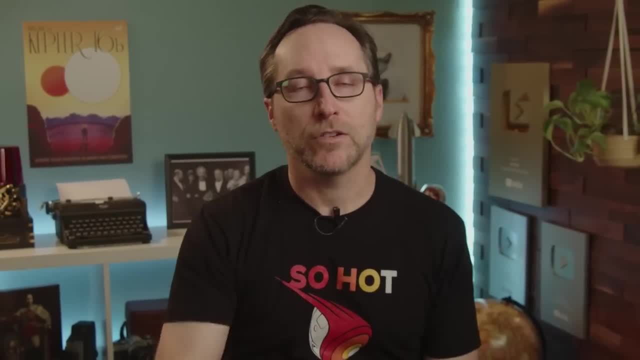 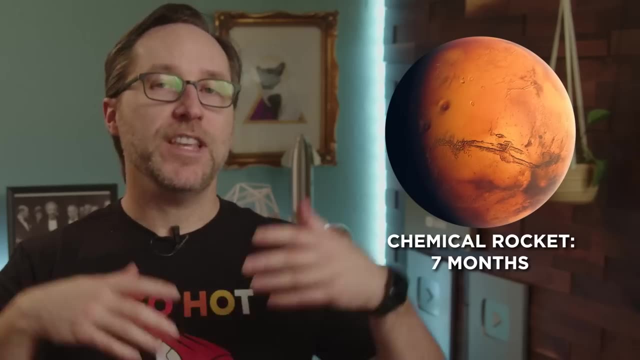 But ultimately, what all that means is that it means we can go super fast across vast distances. There's a reason why they're starting to take this more seriously At the same time that we're making plans to send people to Mars. So, for example, 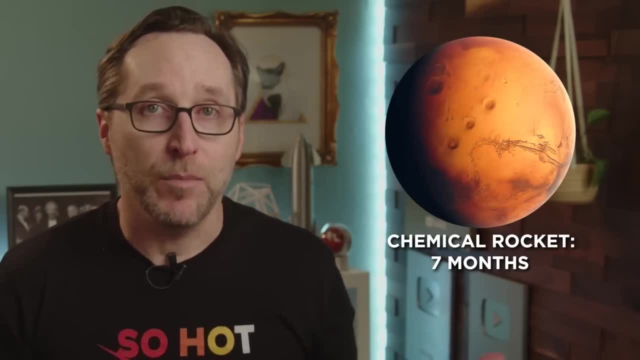 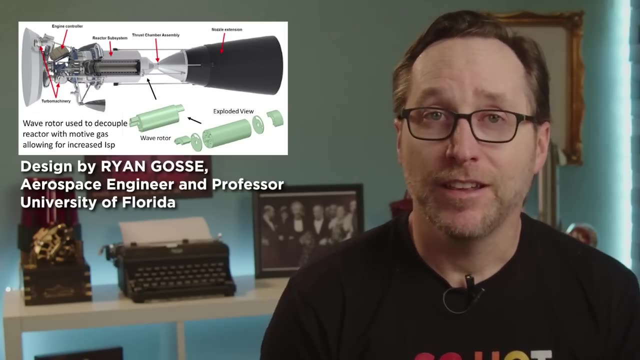 a one-way trip to Mars using modern chemical rockets takes about seven months. A nuclear rocket would make it about 100 days, And at least one new design from NASA could do even better. Just weeks before the Draco announcement, an engine designed by Ryan Goss at the University of Florida claimed to get specific impulses. 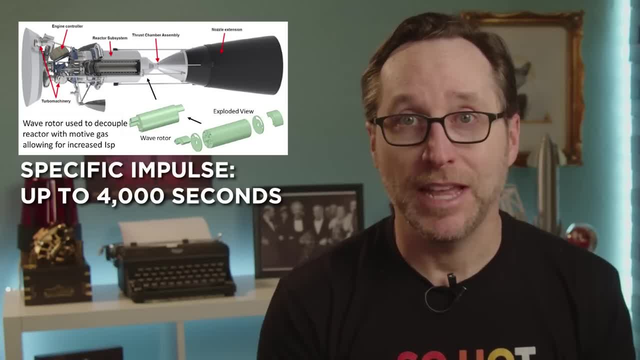 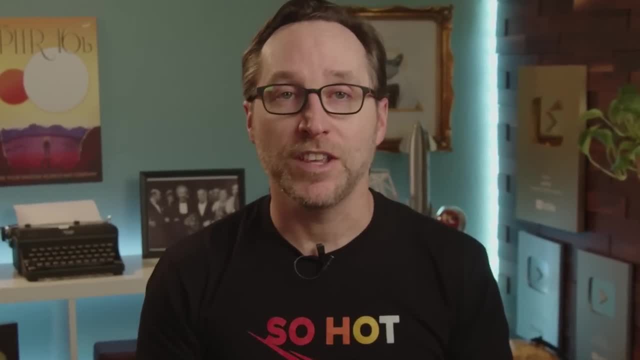 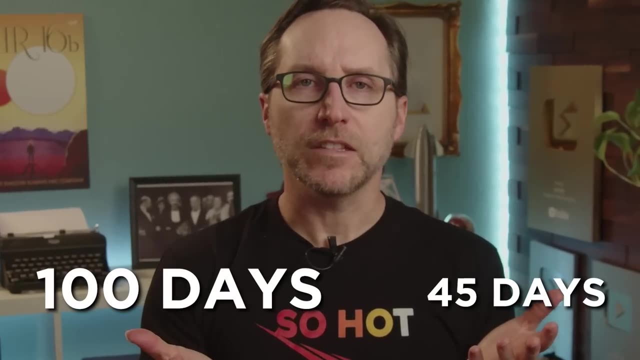 as high as 4,000 seconds, with very little added mass. That's more, A spacecraft powered by Goss's engine could reach Mars in. Are you ready for this? 45 days, That's less, So getting to Mars faster. 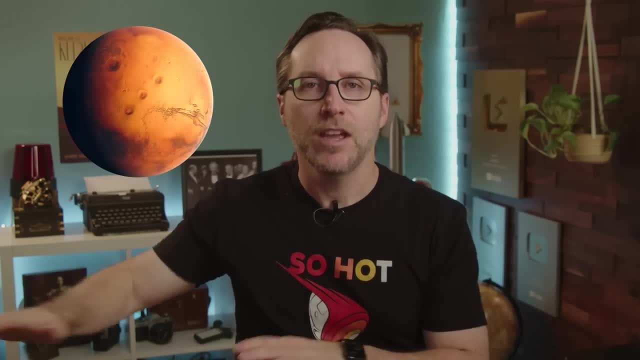 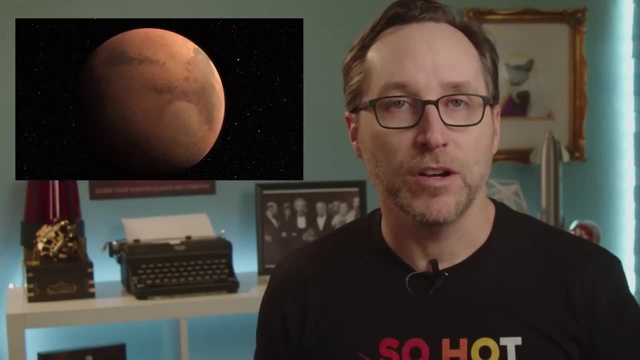 it's not like trying to beat your best time to visit your cousin out in West Texas. okay, Reducing flight time is everything when it comes to Mars. Every single day that an astronaut is spending on the trip to Mars is another day of being exposed to higher than normal radiation levels and cosmic rays. It's yet another day that they're losing muscle and bone density, Not to mention it's an extra day of food and provisions for everyone on board, all of which takes up space and adds weight. Just for perspective, the longest consecutive period any human being has been in space is about 14 months. That would be an average round trip to Mars. So yeah, faster is better for like a million different reasons. So this might be the point in the video when you say: look, if nuclear rockets are so great, why aren't they already in flight? 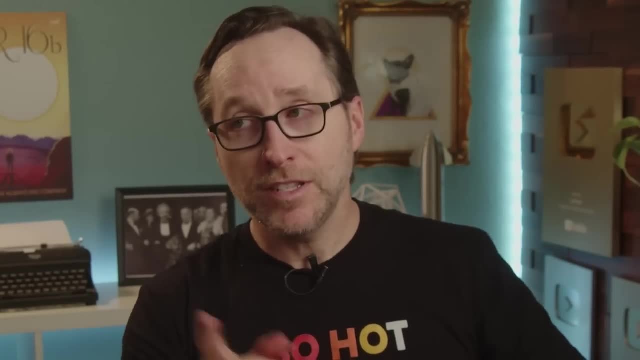 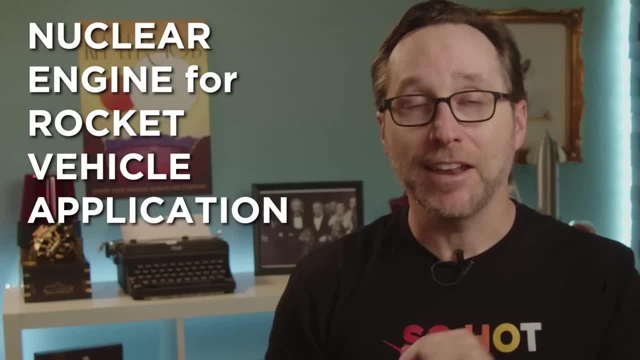 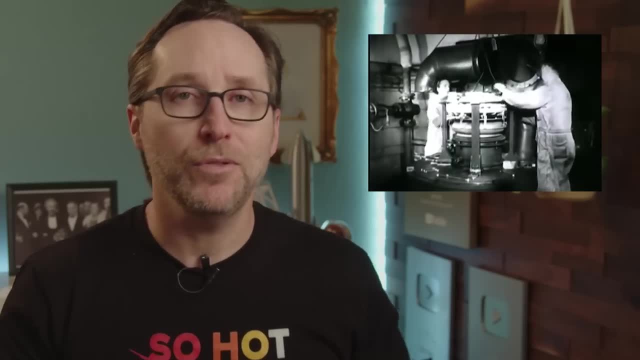 which stands for Nuclear Engine, for Rocket Vehicle Application, And that, kids, is how you acronym. The military had actually been working on atomic propelled spacecraft at the time, because of course they were. The whole world was trying to go atomic at that time. 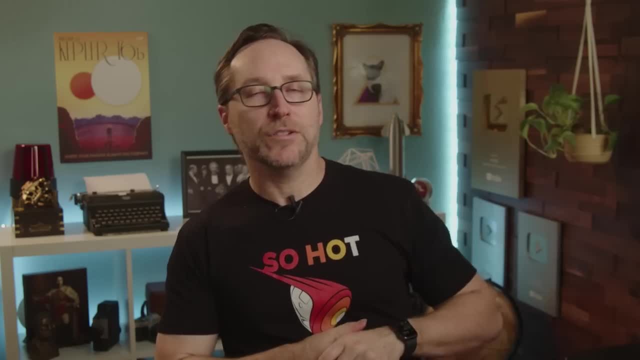 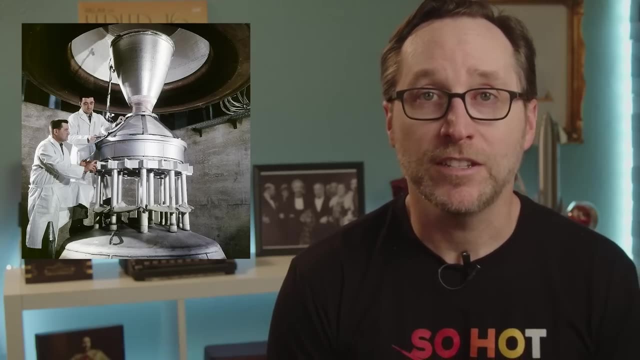 It was the atomic age. But they gave up on those planes because of concerns of the radiation, of course, So they moved on to nuclear rockets. In the late 50s and early 60s several fission reactors for NERVA were built and tested. 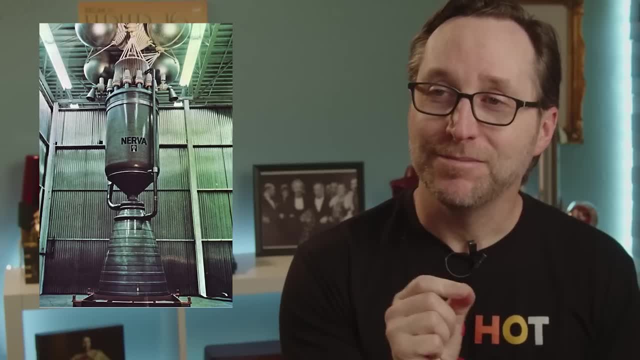 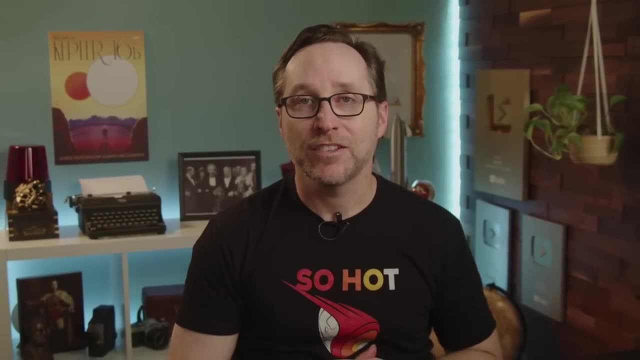 and they got really close to flying, But it never quite happened. I did a video a while back about NASA's original post-Apollo plans, drawn up by the Space Task Group that Richard Nixon had created, which, by the way, if you haven't seen that, it's definitely worth a watch. 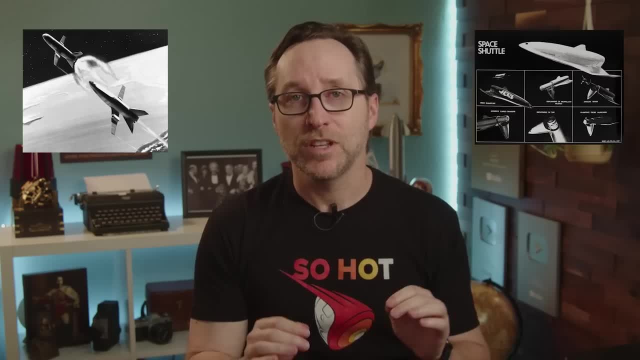 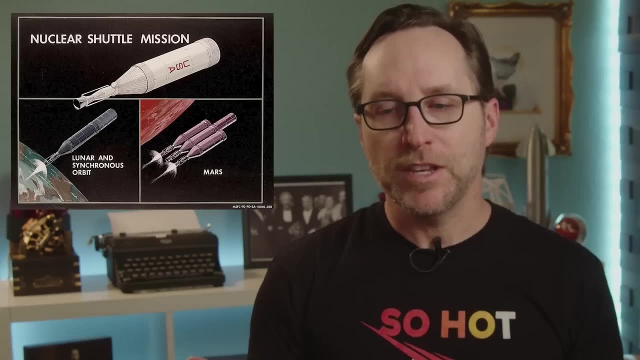 It blew my mind. Some of the plans that they drew up for the 70s and 80s were just kind of bonkers in hindsight, But a lot of it actually relied on this NERVA engine. Yeah, they had plans for nuclear spaceships that would carry people and cargo. 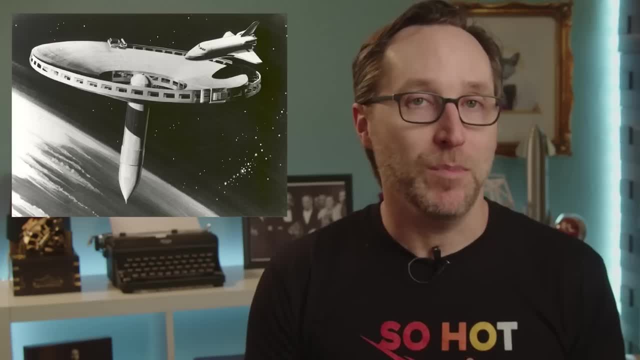 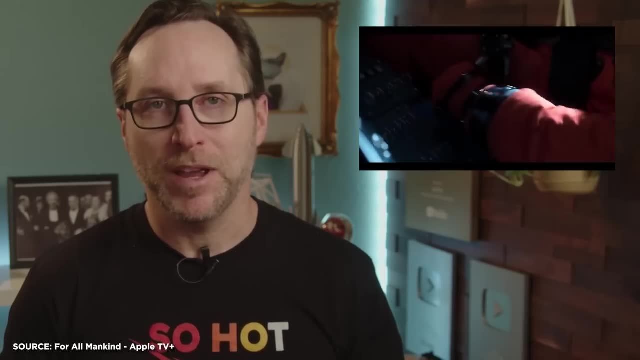 in between all the different, various space stations around the Moon and around Earth and the Moon bases and stuff like that, all of them powered by nuclear engines. Also, fans of the Apple TV series For All Mankind might know that the NERVA engine 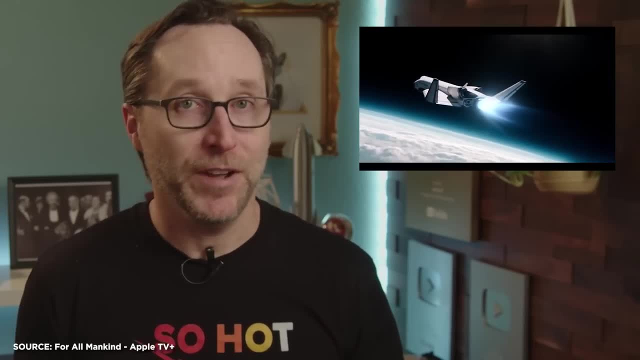 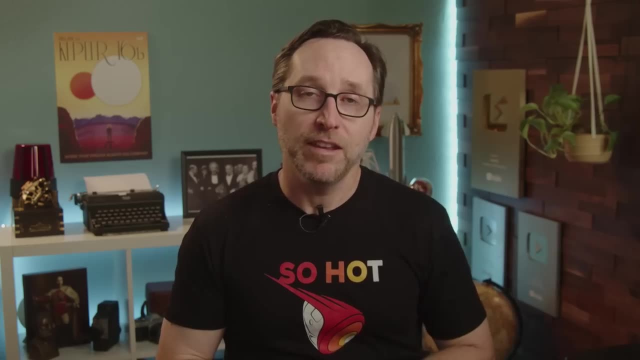 was actually what they put on their version of the space shuttle, which they call Pathfinder. But anyway, in 73, when Nixon was president, the Apollo program was winding down and, yeah, a lot of programs got cut and NERVA was one of those programs. And in a bit of a double whammy, the Soviets were actually working on their own nuclear rocket at the time, and when they saw that the Americans cut their program, they kind of just, you know, let their slide aside. It really was just a big pissing contest. 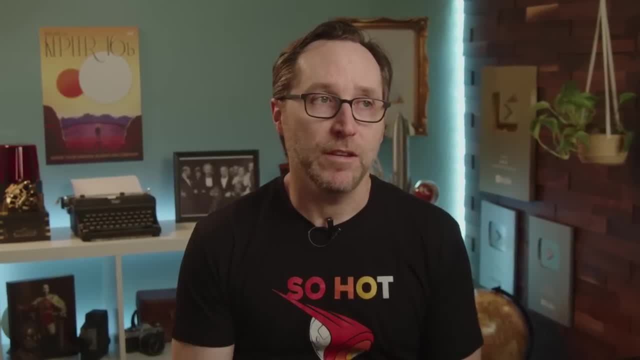 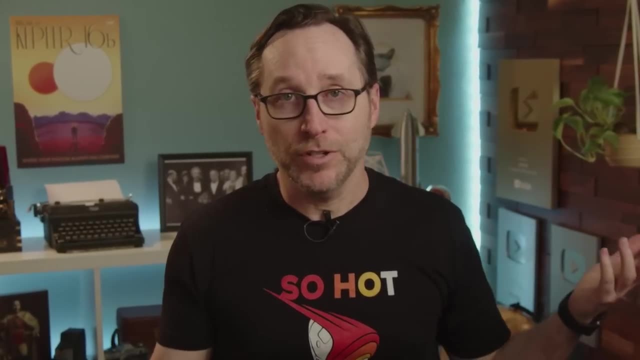 But probably the biggest thing holding back nuclear propulsion is the environmental question. I mean, we are, after all, putting nuclear reactors on top of massive controlled explosions. Now, to be fair, the NERVA program actually had an incredibly good safety record. 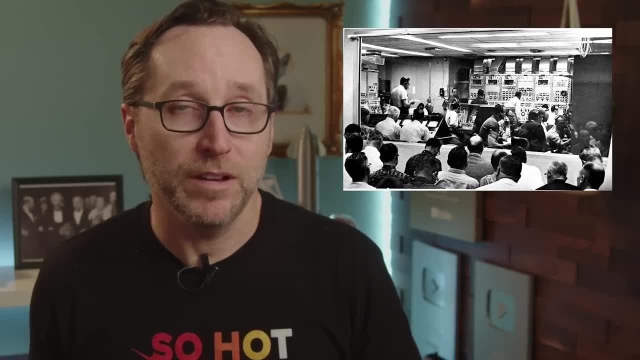 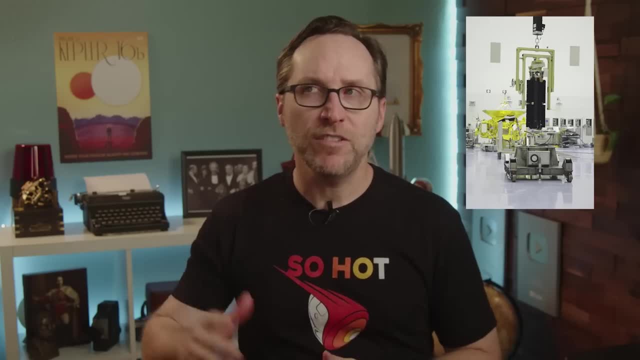 and space programs have been launching nuclear materials since 1961, usually in the form of radioisotope thermoelectric generators or RTGs. These provide power for satellites and space probes, especially if they're going really far into deep space where solar energy is harder to come by. Between 1961 and 2006,, the US successfully flew 41 RTGs to space. Those include the New Horizons spacecraft in 2006,, the Curiosity rover in 2011, and then 2020,. the Perseverance. They haven't all gone perfectly, though. For example, in 1964, a US launch failed, resulting in a small amount of plutonium-238 being released into the atmosphere. Plutonium-238 isn't great for humans, especially the skeletons and livers which, according to Wikipedia, are important. 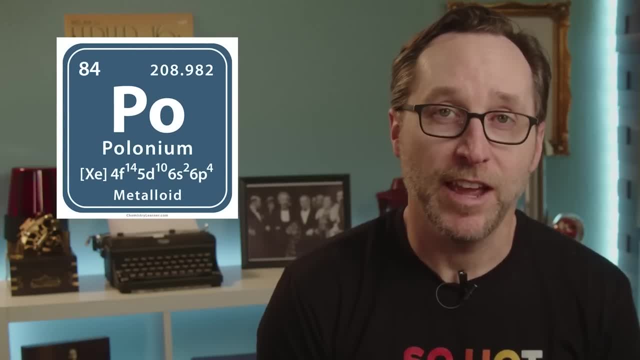 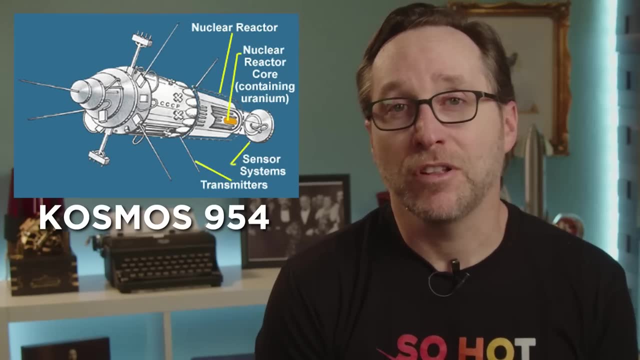 A large section of Russia was showered with plutonium in 1969, and in 1978, the loss of the USSR's Kosmos 954 satellite caused uranium to fall down on a 600-kilometer swath of Canadian soil. The Canadian government charged Russia with $6 million for the cleanup. They eventually collected about half that much. The point is, we've actually been launching nuclear material for a long time. Uh, yes, there have been a few issues, but nothing bad enough to ban them. Also, rocket safety's come a long way since the 60s and 70s. let's be honest. 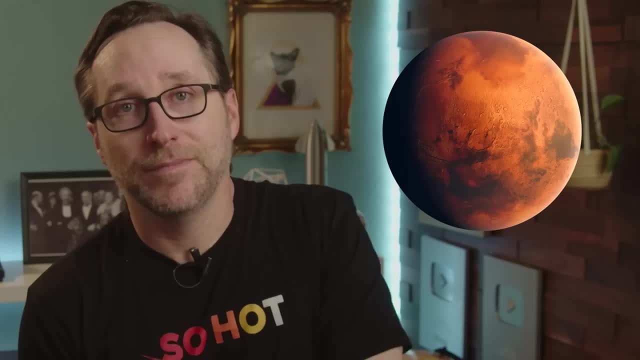 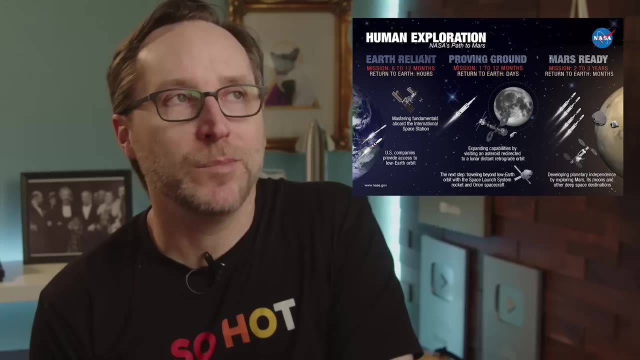 So I, for the record, am excited about this. I really think that if we're going to get serious about going to Mars, if we're going to get serious about going, you know beyond, as NASA keeps saying, with the Artemis program, 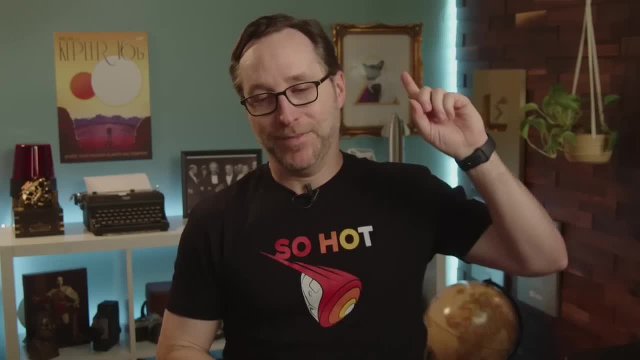 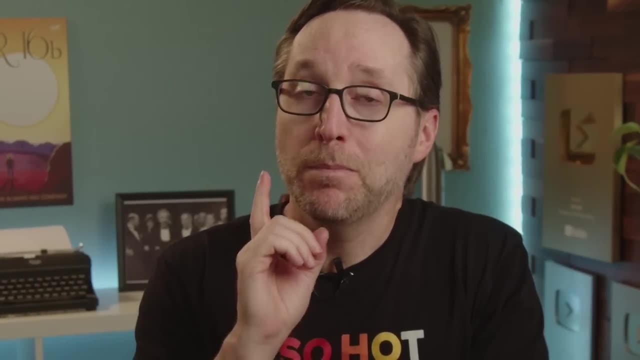 then we're going to have to get serious about nuclear propulsion. But if we really want to go beyond, there's something beyond nuclear thermopropulsion and that is nuclear pulsed propulsion. Sounds similar, It's very different. 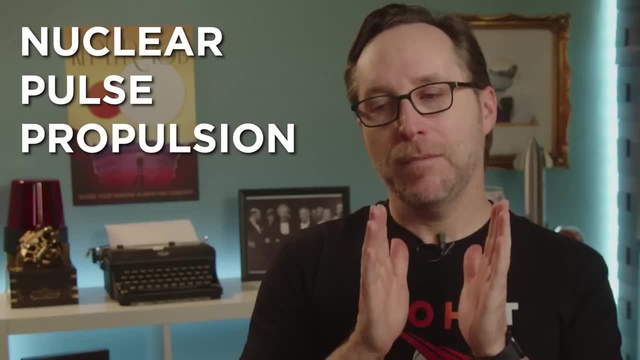 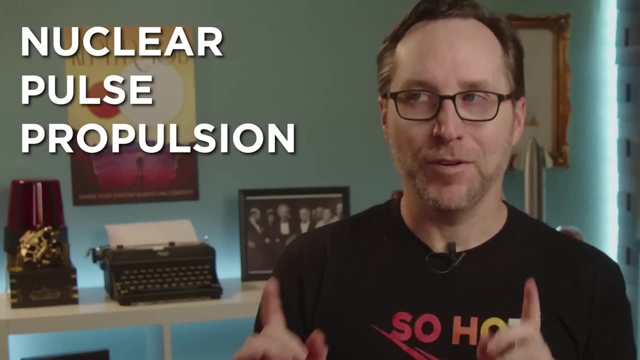 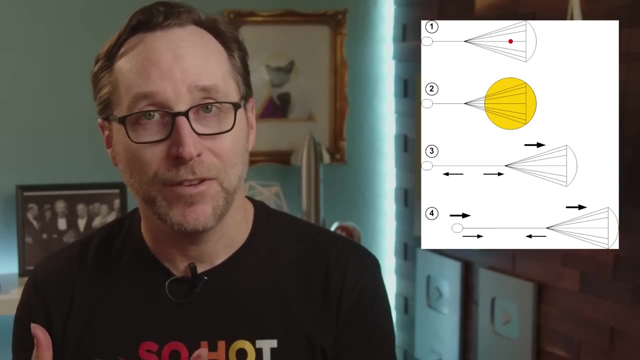 Nuclear pulsed propulsion is basically pushing a spacecraft forward by setting off nuclear explosions Over and over and over again. Yeah, that's the pulse. So the shockwave from this explosion impacts a pusher plate and then the spacecraft moves. Now, as you can imagine, you can get some pretty high-specific impulse and speed. from straight-up nuclear bombs going off by themselves, off behind you. How high? Well, the US actually developed something like this. They called it Project Orion and it was expected to achieve 6,000 seconds on the low end to 100,000 seconds. 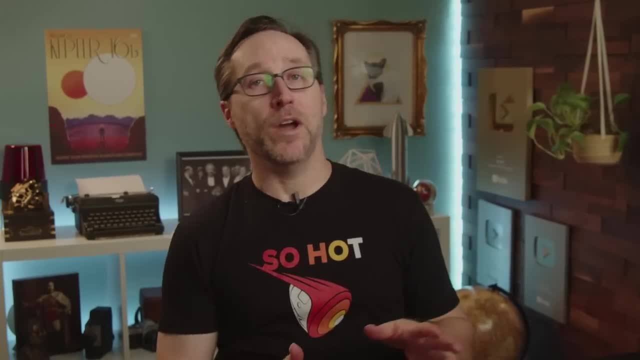 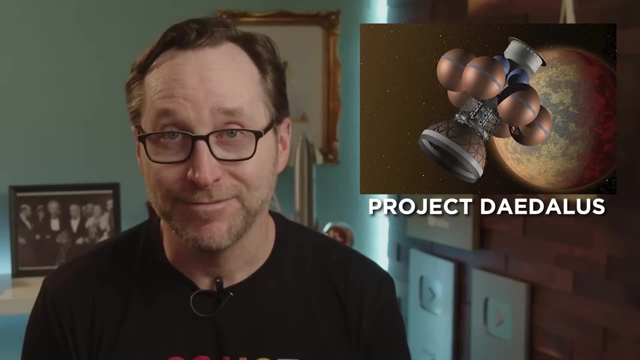 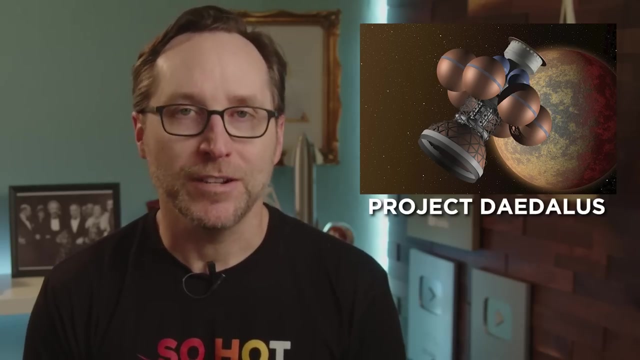 on the high end, 450.. Even more bat-guano crazy was Project Daedalus, which was proposed by the British Interplanetary Society. It proposed speeds equal to half the speed of light, But big caveat here- it would require fusion power. So yeah, it was a bit more of a thought. 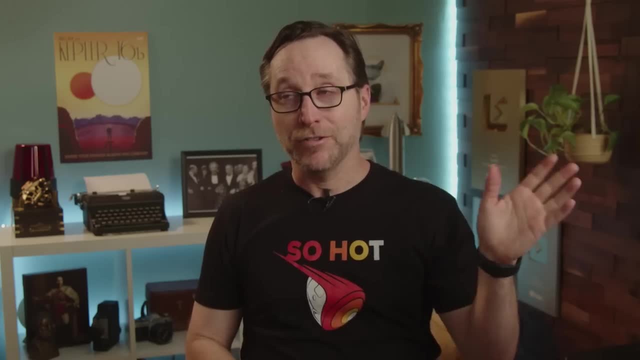 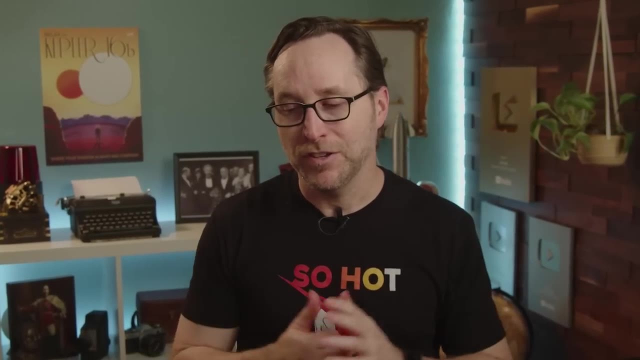 experiment. Just to be fair, though, if we ever were to get serious about interstellar travel, we would need exactly something like that. The only problem with Project Orion is that, and pulse propulsion in general is that, if we were to ever try to really 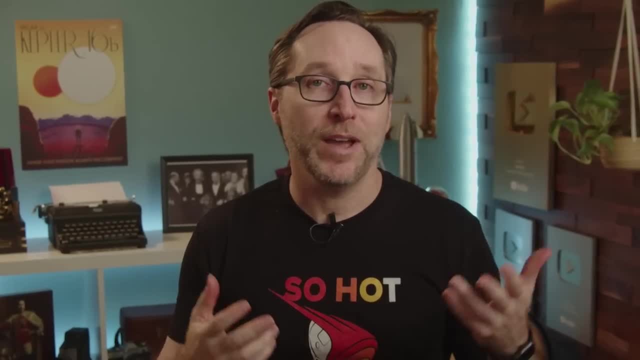 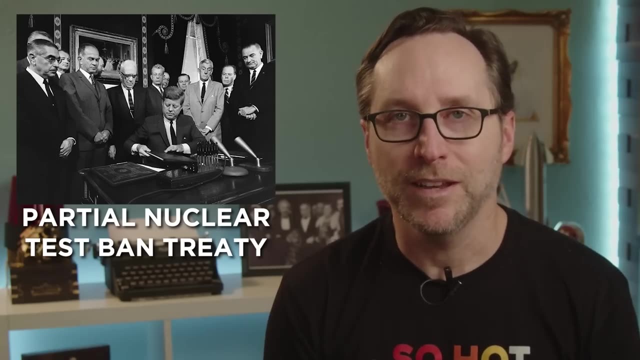 explore that we would have to actually re-evaluate our international nuclear treaties. Yeah, the Partial Nuclear Test Ban Treaty of 1963 was one reason why Project Orion was abandoned. Kind of hard to test out that rocket without setting off some nuclear explosions. 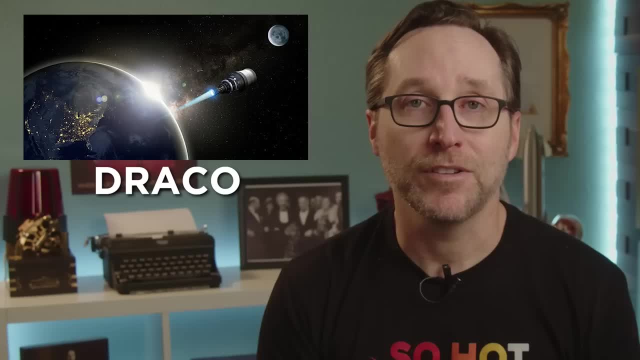 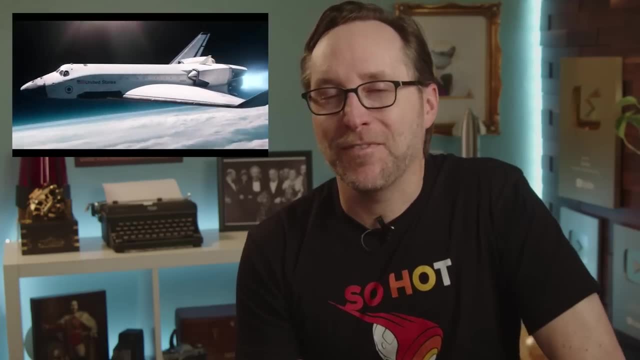 But hey, Draco seems Seems to be a great first step, And I do think their timelines are a bit ambitious, but I'm excited. I'm looking forward to seeing what they come up with. I want to see something like the Pathfinder from For All Mankind. 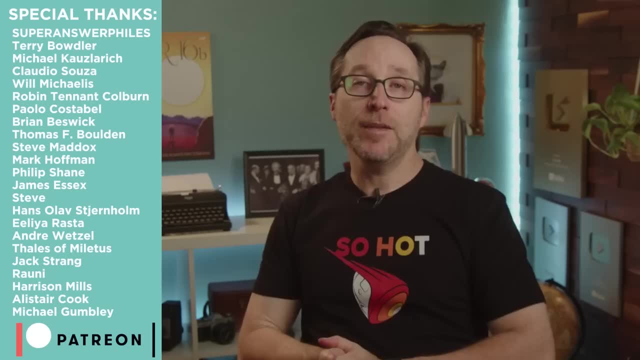 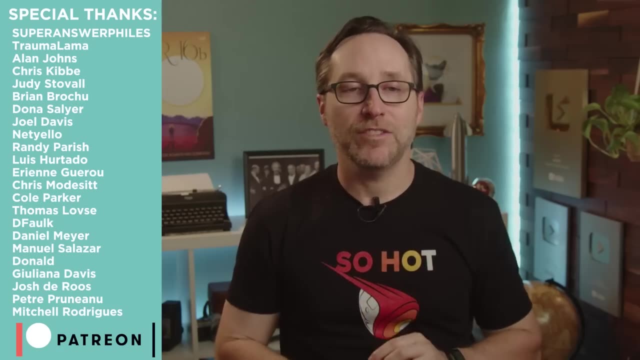 I do. That was badass, All right, so hang tight, because in just a minute I'm going to give the update on the winners of the sketch round from last week. Some exciting stuff there. but real quick, let me shout out some new channel members. We've got Laura Sosa. 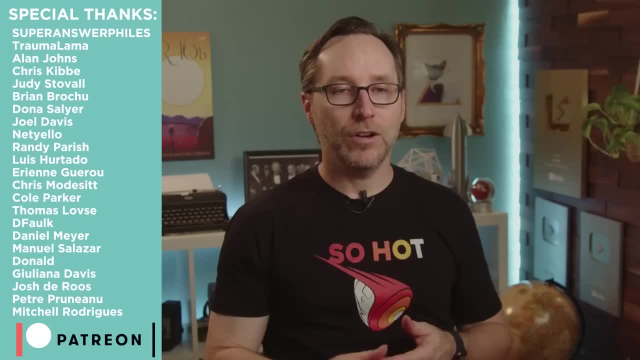 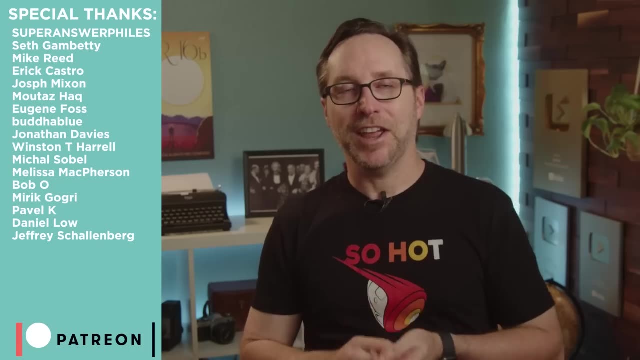 Gator Livius, Vicarious Traveler, Joe Grosel, Carter Wolf, Christopher Thomas, Jeff Bryant, Riley, Family Friendly Fun. Michael W Miller, Will Frank and Jason Kay. Thanks to you guys so much. These are channel members. These are people who are contributing some amount of money to help keep. 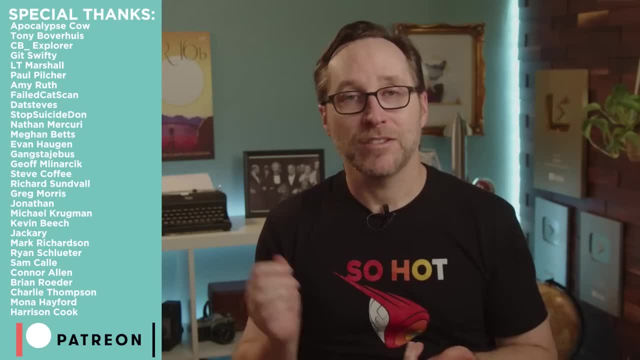 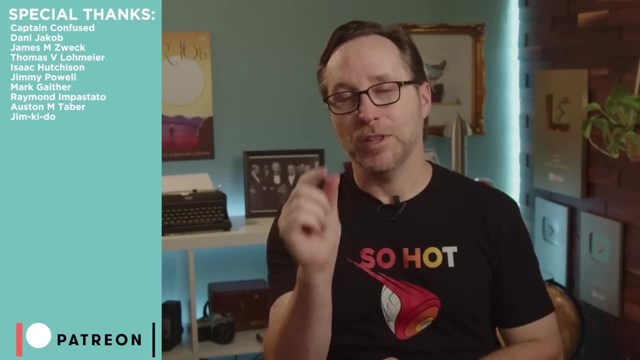 the channel going, which I do appreciate, And in return they get perks like exclusive live streams, early access to the videos and all kinds of other cool stuff. You can see them in the comments down below, with little things next to their face. If you would like to be one of them, just hit the. 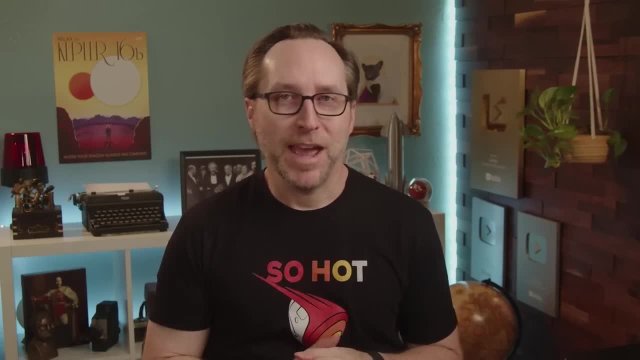 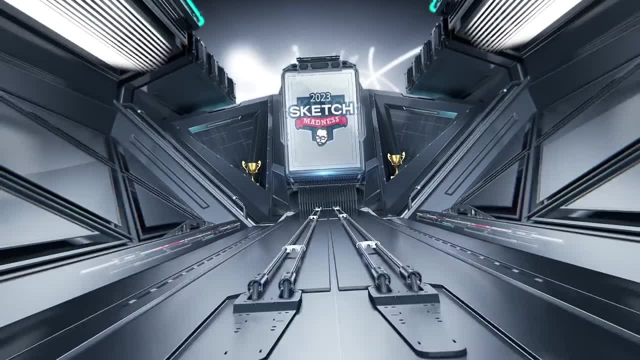 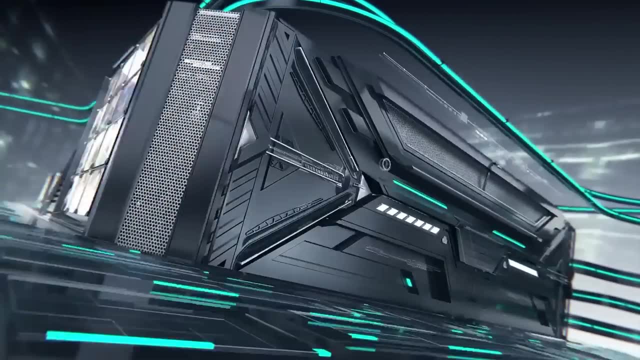 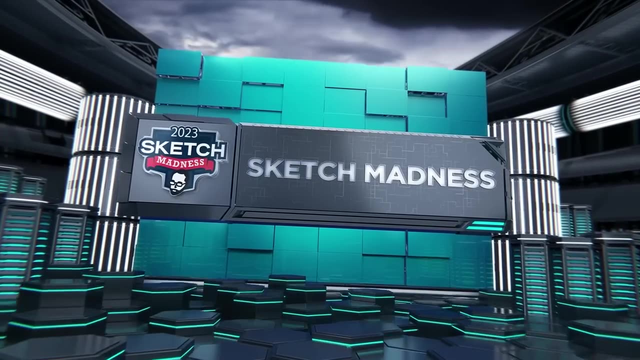 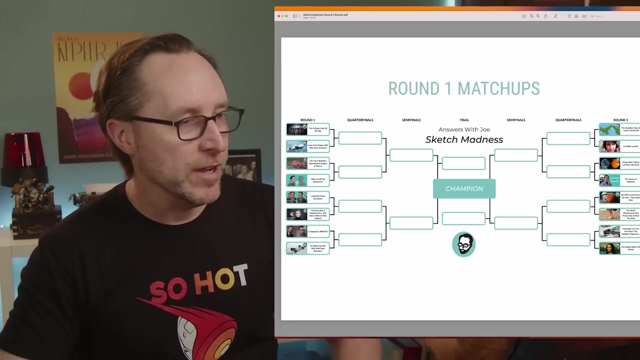 So here's today's Sketch Madness update. Okay, I decided I would do a blind reaction to the results, so I haven't seen these yet. So here's the full brackets. Here's what you guys voted on. First matchup was the five worst cults of all time versus how Crew Dragon will help open up space. 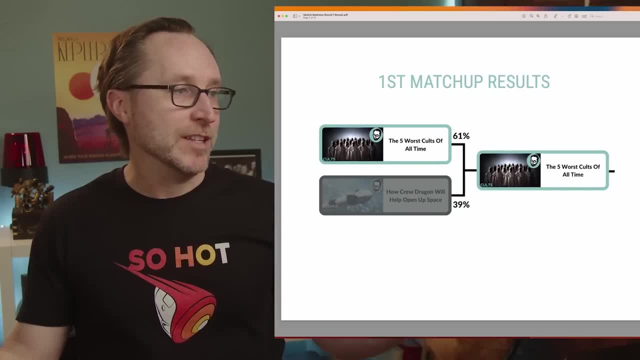 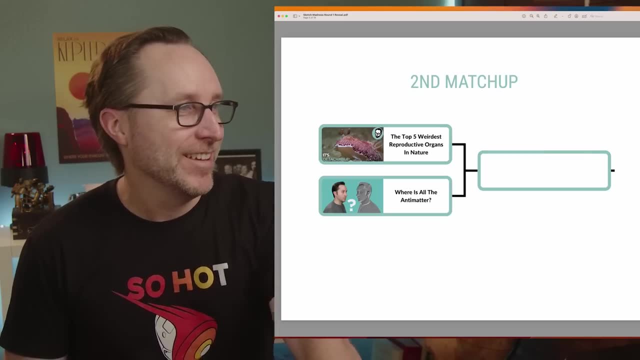 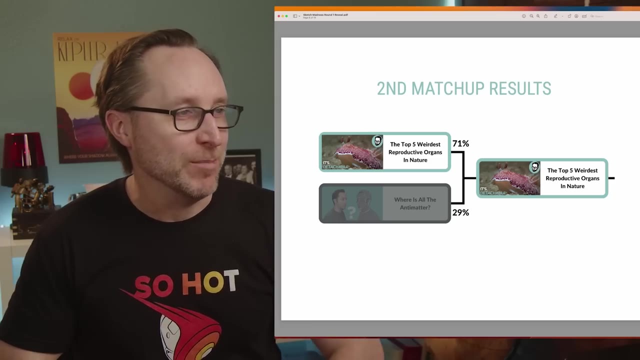 The winner was five worst cults of all time, with 61% of the vote. That was closer than I thought it would be honestly All right. next matchup between these two Yep Penis Designer. Okay, this is about what I expected, But anyway, 71% versus 29% on that one. Next up, drum roll, please. 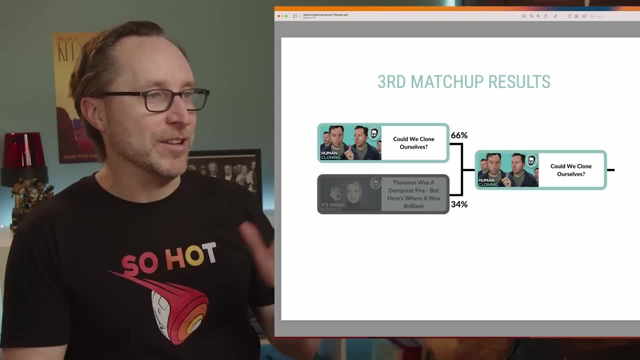 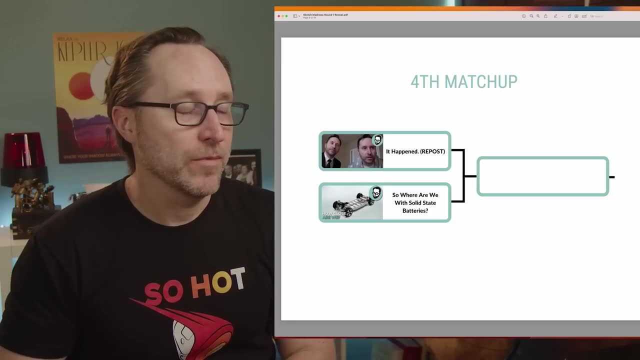 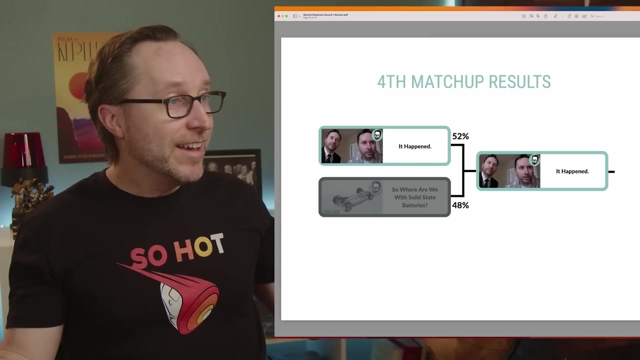 The winner is, of course, 66% to 34%. Again, kind of surprised that one was so close. Next matchup: this was the 1 million subscriber celebration video. I know which one's gonna win this one. We all know which one's gonna win this one. Hey, look at that. What? How is it that close? 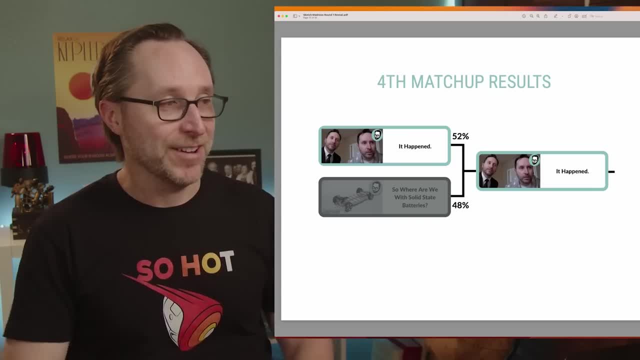 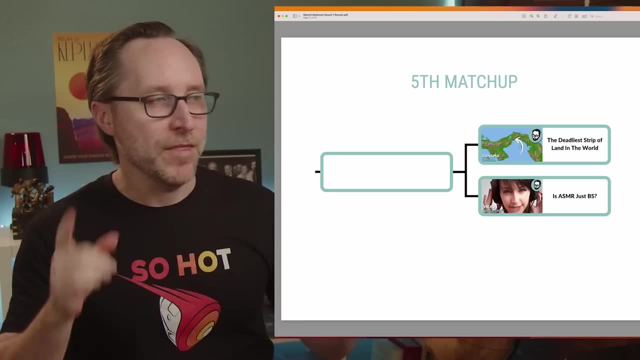 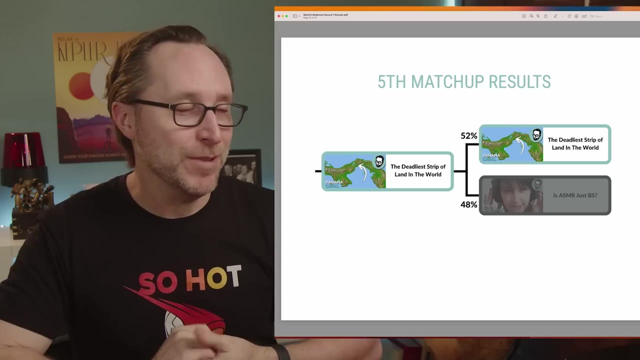 This is the biggest surprise so far for me. Wow, Okay, so 52 to 48, but the one that won is the one that I thought would win All right next matchup. I think I know which one. this is gonna be Also very close, Okay, wow, I really thought that wouldn't would be. 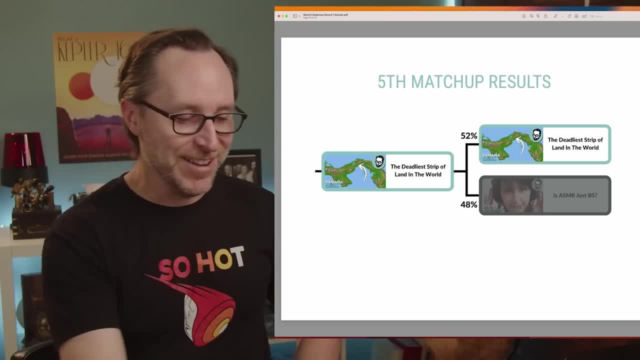 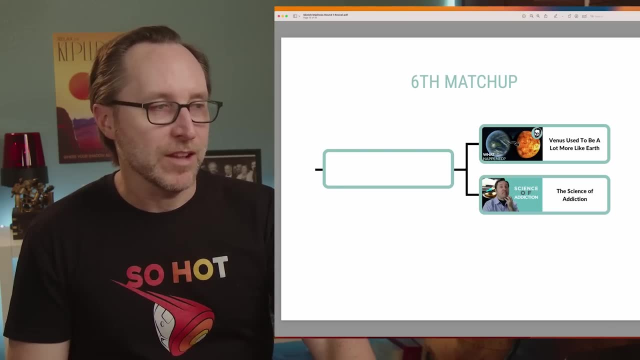 Uh, blow it out of the water. Okay, well, let's keep going. The Venus one was fun. We had some cool like makeup effects and stuff. but I think the Science of Addiction one's gonna win and the winner is. 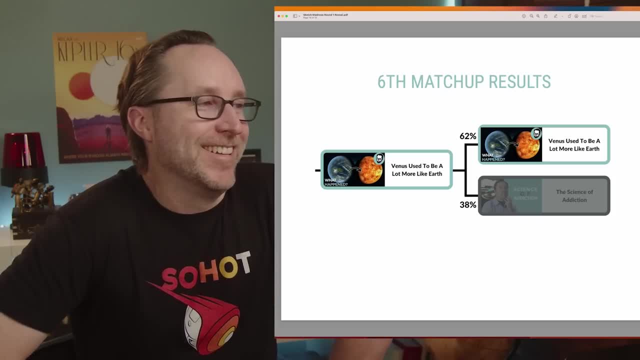 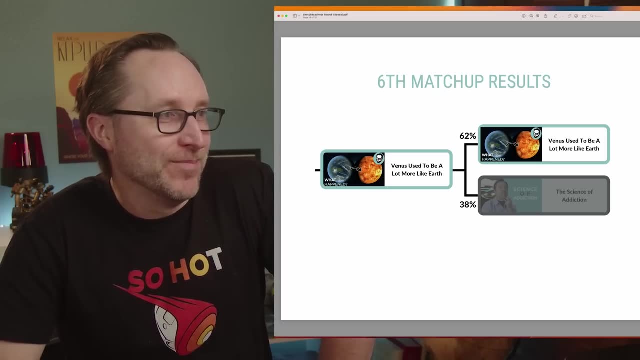 What? Okay? Well, I'm out. I wouldn't have gotten that. I really thought that the other one would have gotten better. Let's go on to the next one. I'm pretty sure I know which one. this one's gonna be The first one. 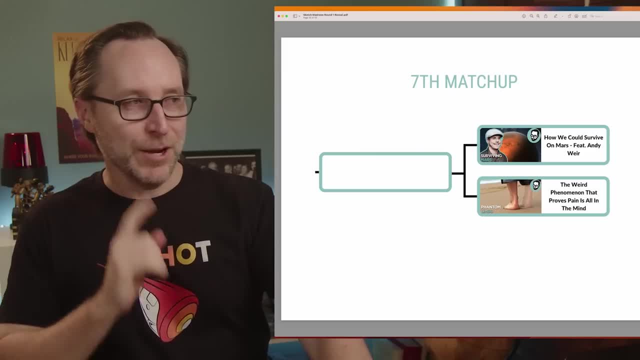 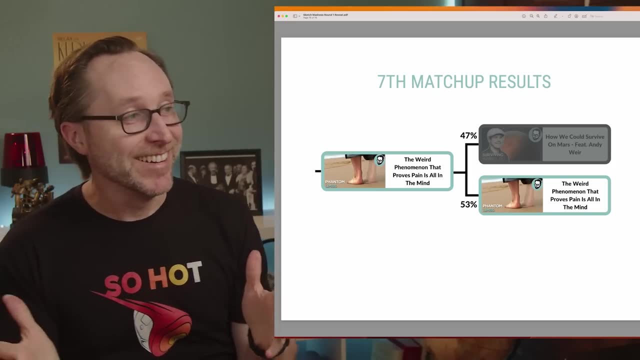 I actually Got Andy Weir involved. I think I know which one's gonna win this one, and the winner is: Oh my god, what an upset. There's been some upsets here. Okay, 53 to 47.. That one's the winner. All right, last one. 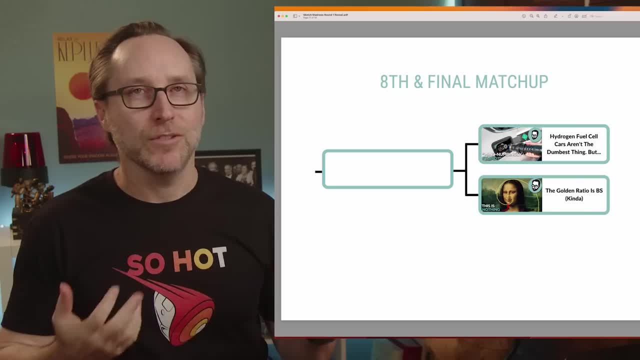 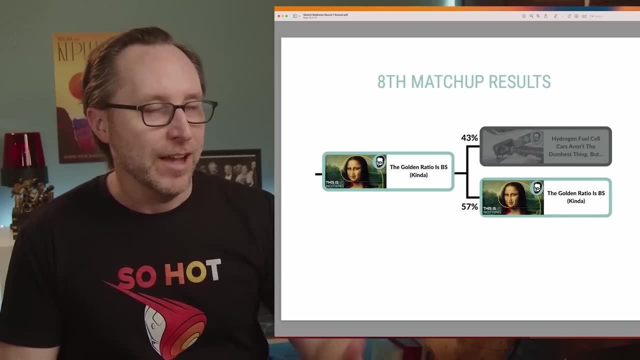 Uh, hydrogen fuel cell versus the golden ratio. The hydrogen fuel cell one. I actually That one has Zoey in it. I think that's gonna be the winner here. Let's see: No, No, No, No, No. 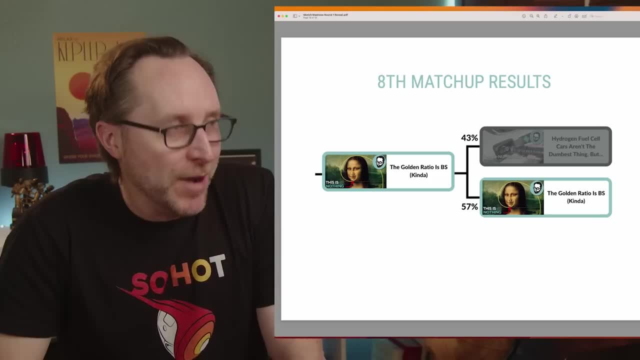 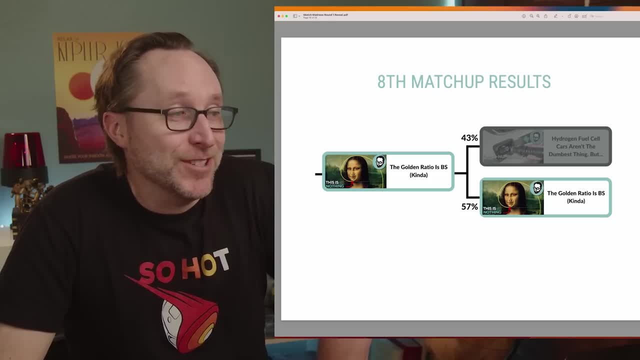 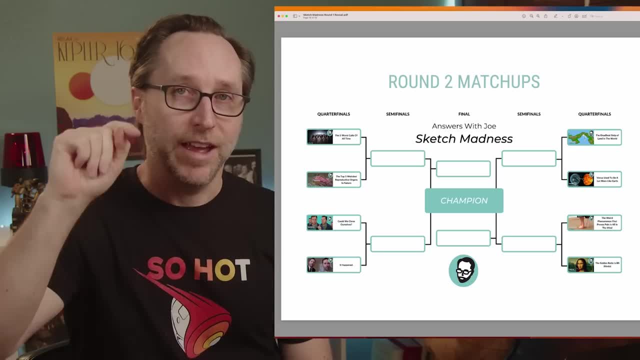 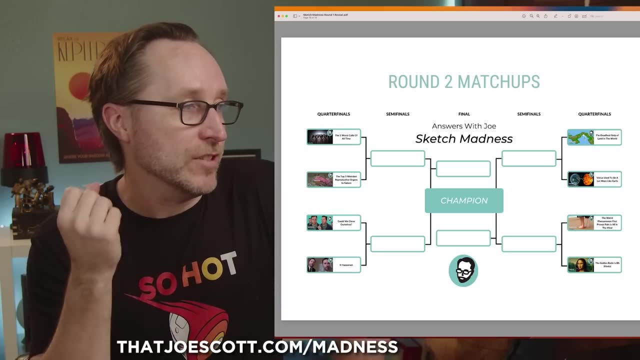 Round two is now live as I speak on the website That is thatjoescottcom. madness, Go there to vote for these. You got the worst cult of all time versus the top five weirdest reproductive organs in nature. Could we clone ourselves? versus the second clone. 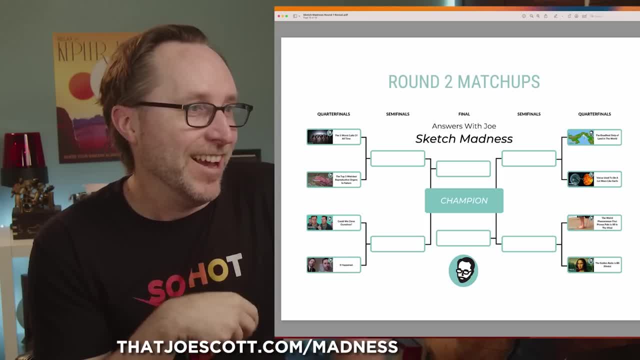 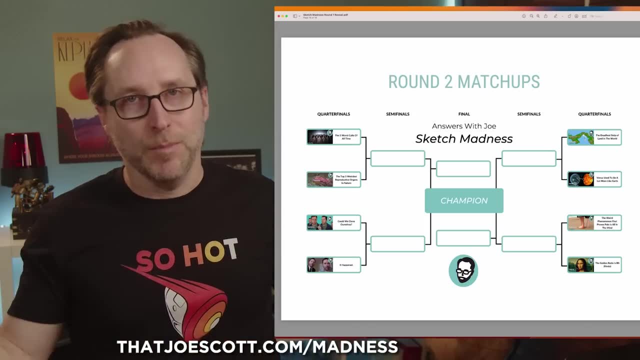 So these are the two clone videos going up against each other. That's going to be interesting. The Deadliest Strip of Land in the World versus Venus Should Be a Lot More Like Earth. And the Weird Phenomenon that Proves All Pain is in the Mind about phantom pain, basically. 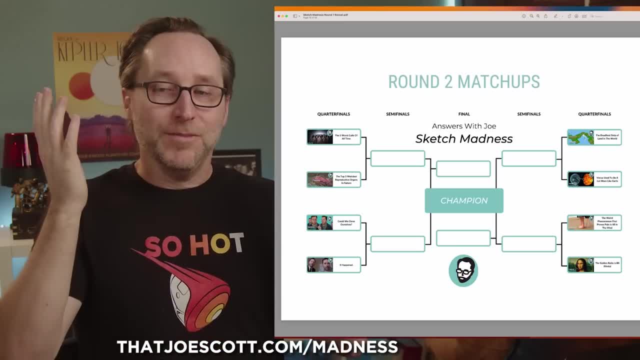 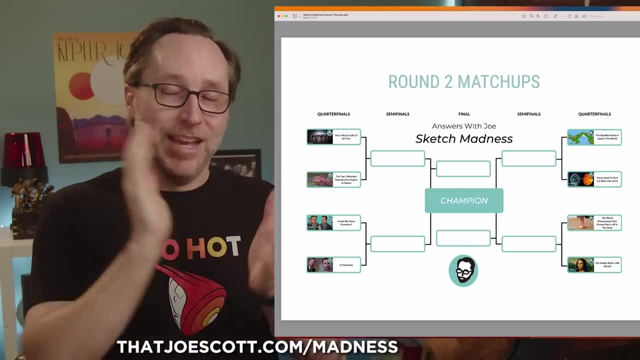 And the Golden Ratio up against each other. So you guys have really surprised me This, really. There were some upsets here for me, honestly. So go there to thatjoescottcom madness, Vote for this next round, and you're going to surprise me again. I feel like